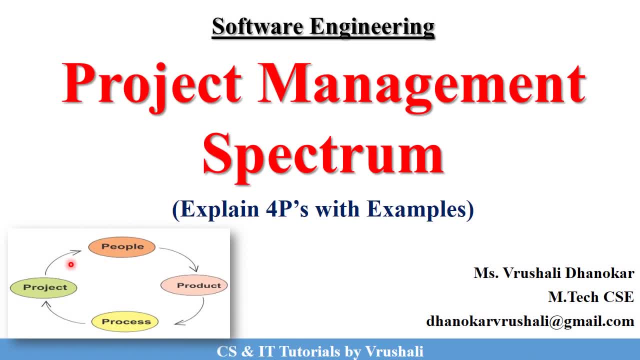 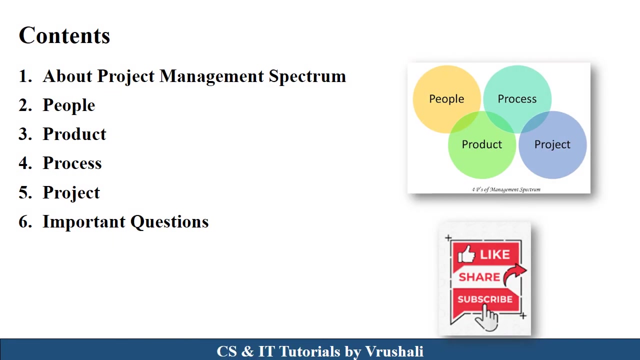 Hello everyone. this is Vrishali. In previous session we discussed about project planning process and project scheduling with examples. I have mentioned complete software engineering subject playlist link in below description box. Now in today's session we will discuss the next important topic, that is, project management spectrum. Let's start the session. 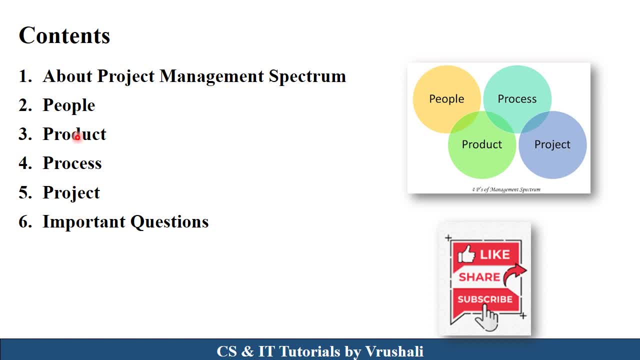 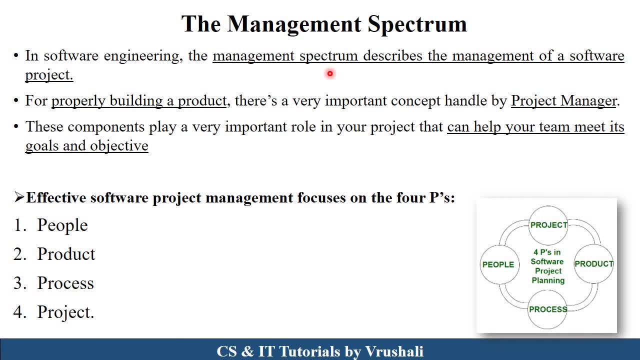 In this session we will discuss all four project management spectrum with examples and some important questions that have asked in previous year question papers. Now the first thing is: what exactly management spectrum? In software engineering there are four P's, which is called as management spectrum. They describe complete management of software. 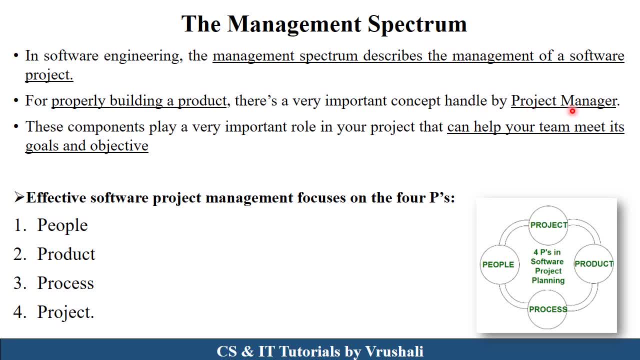 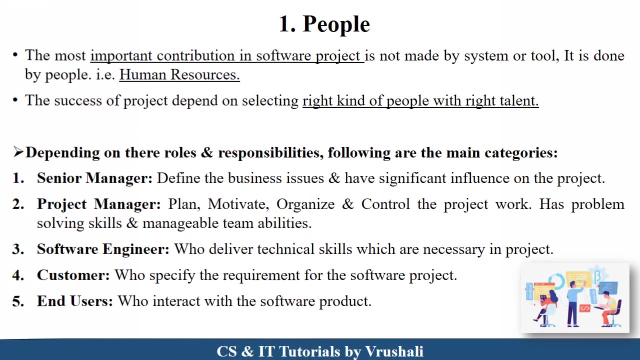 project. This spectrum are handled by project manager in planning phase of software development life cycle. For effective software project management there are four P's like people, product, process and project. This all components are play very important role while developing a particular software project as per the customer requirement or customer objectives. 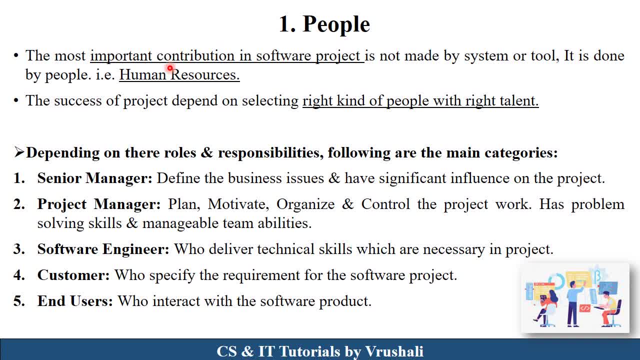 The first P is people. In software engineering, people, or human resources, are the most important contribution for software project. The success of project is completely depend on selecting right kind of people with right talent. In software engineering, there are various roles and responsibilities. Following are: 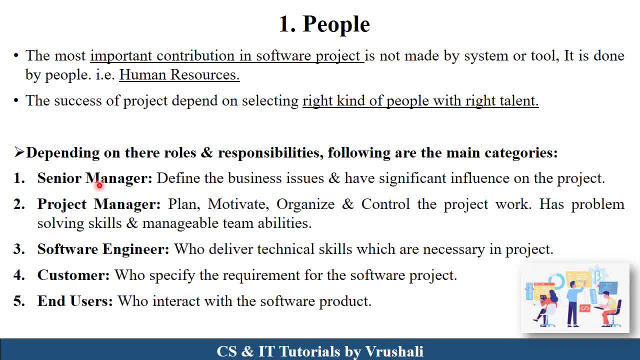 the main categories. The first one is a senior manager. Senior manager define all the business issues and business problem that have significant influence on particular project. Project manager: plan your complete project, motivate all the stakeholders, organize your project and control your complete project work which has a problem-solving skill and manageable team abilities. The next one: 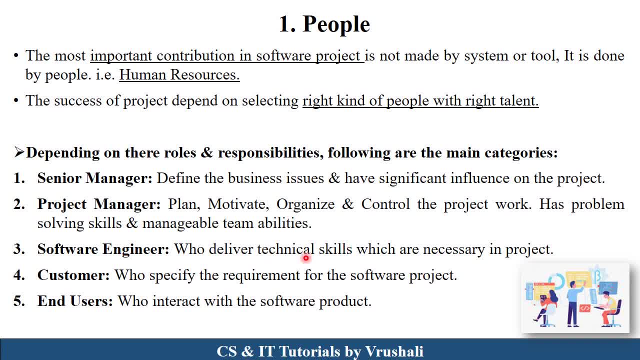 is a software engineer: Software engineer who deliver all the technical skill which are necessary for particular project, Which include all the designer, developer, programmer, tester and all the technical person. The next one is a customer- Customer having the highest priority in software engineering, Who specify the complete requirement of particular software project. 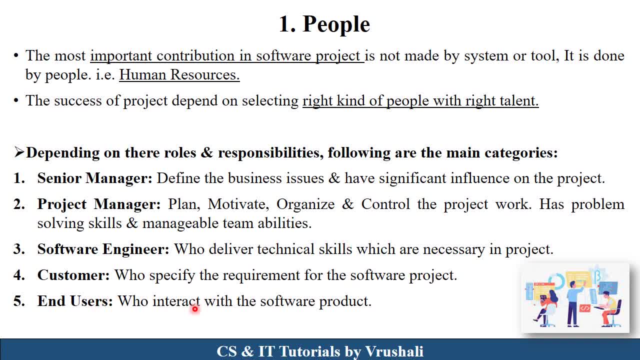 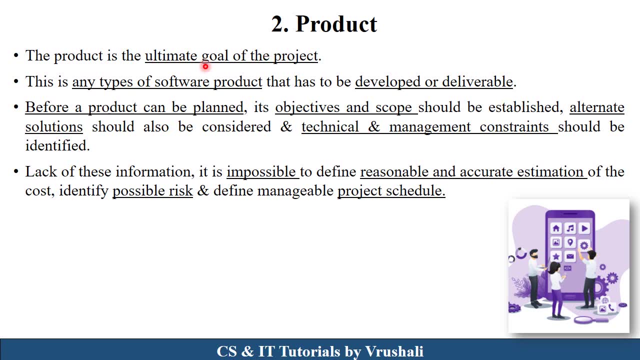 The next one is the end users. End users means who interact with all the software product, Who use all software products, So people and human resources having important role in software engineering. Now the second P is product. Basically, product is a ultimate goal of your project. There are various types of software products. 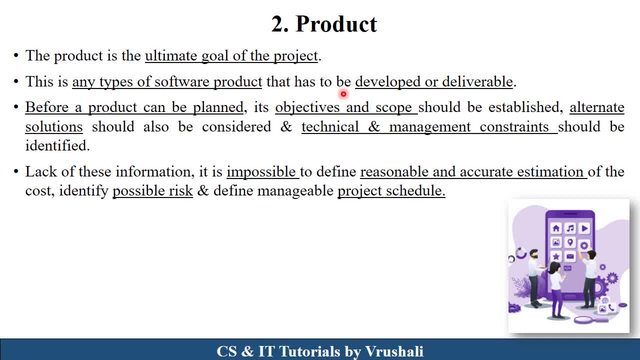 Like web development product. Then app development is there, Hardware development is there, So which is called as product. But before starting a product development, Every stakeholder must know objective and scope of particular project. There are various types of software products. There are any alternate solution regarding particular design and development. 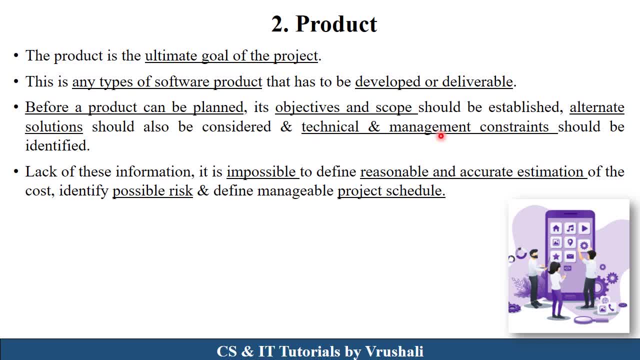 Some technical and management constraints, Some software and hardware resources Before development. you must know all this thing, Lack of this, all types of information, So which is very impossible to develop this project As per the cost, as per the timeline. So that's why product play a important role. 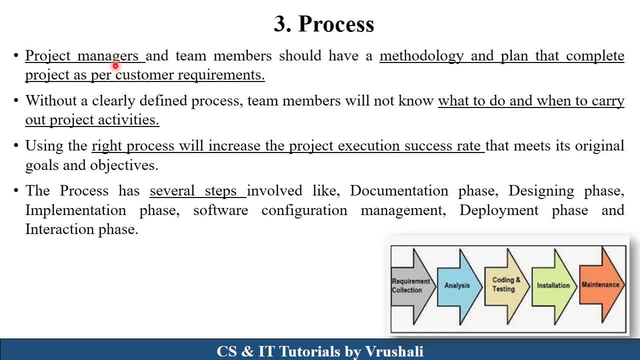 The next P is process. So here project manager, define various methodologies and plan To complete a project as per the customer requirements. As we discuss, in software development life cycle There are various process like requirement gathering and analysis, Then planning, coding, testing, installation, maintenance. So this, all phases are called as process. 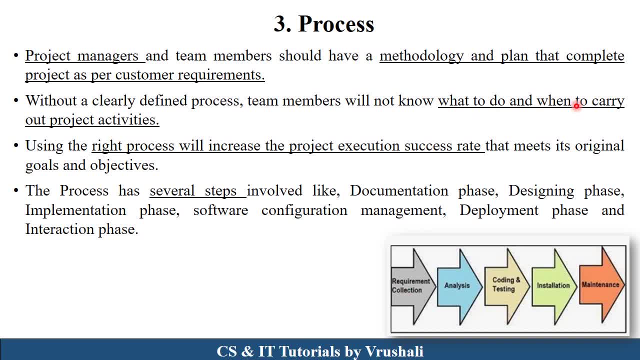 That's why stakeholder must know what to do And when to carry out all the project activities. Using right process will increase project execution success rate. That's why this all process will be used to create project success rate. This all process are important. This all process performs sequentially. 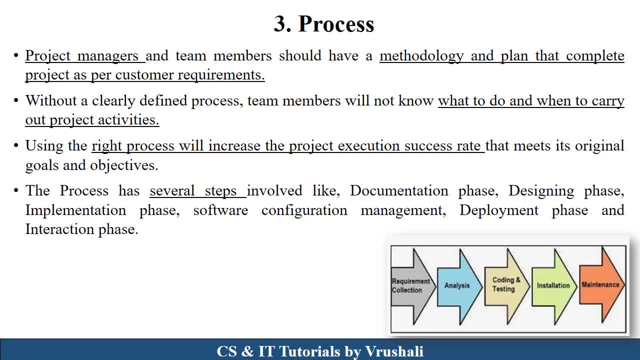 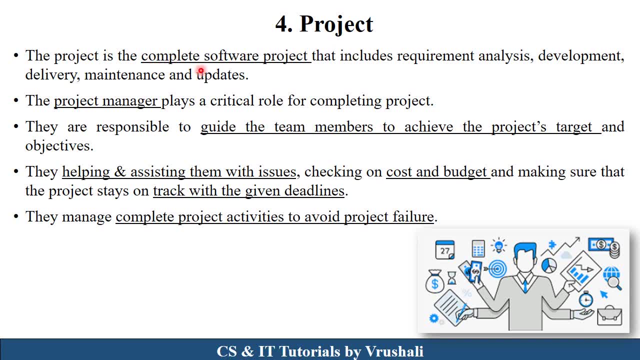 They send input and output to with other. Now the next P is project. So basically, project is a complete software project. When you perform all the process, From requirement gathering, analysis, Planning, designing, development, testing, After that maintenance and all the updates, This all process have performed. 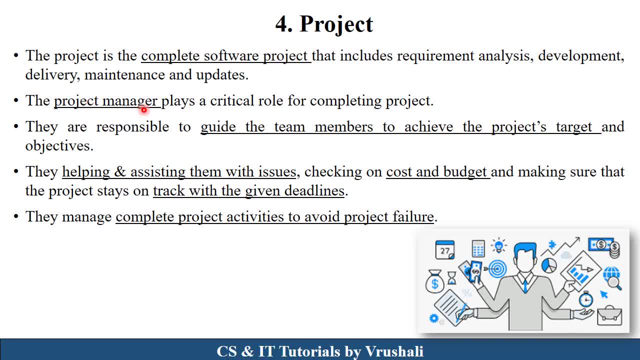 And after that your projects have generated. So project manager play very important role for completing your project. Project manager is responsible for guide all the team members To achieve project target as per the customer requirement. Project manager help and assist them With all the issues and problems have occurred.